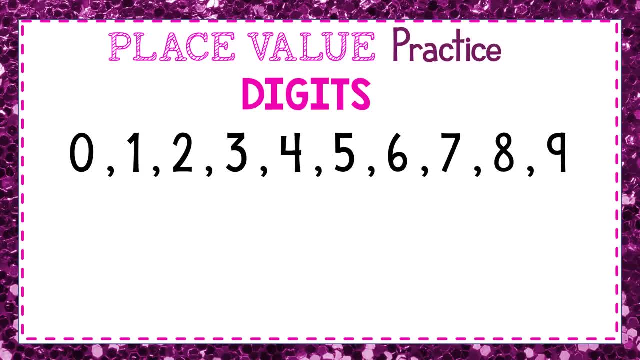 number that you and I may see, read or write in our counting system. For example, if I have a 2,, that represents just 2.. If I have a 5 and a 9,, I can make 59 or I can make 95.. 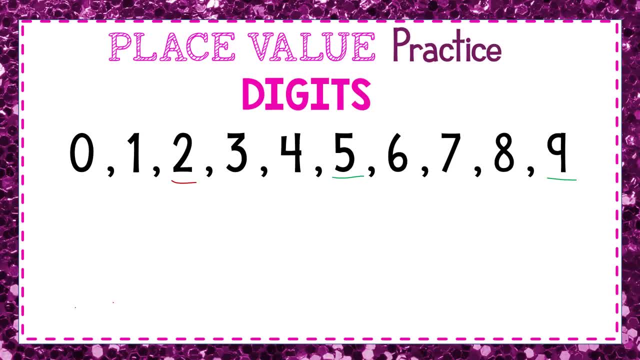 Every digit here can create the biggest number or the smallest number. If I wanted to make the number 9875 432, I've used almost all of my digits and I've made a 7 digit number. so digitsக 4,. 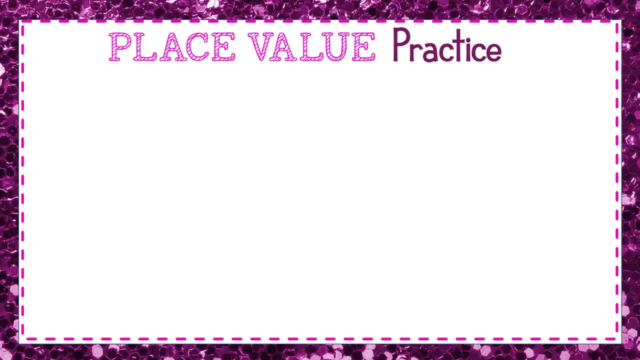 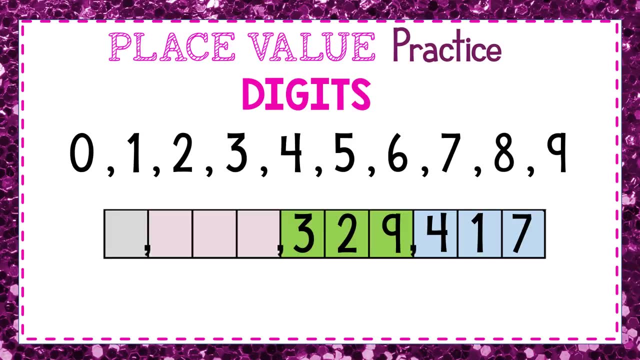 5, the numbers that we use in our counting system. so let's look at a number in standard form. here I have the number three hundred twenty nine thousand four hundred seventeen, and let's look at the digits that make up this number. as you can see, I have a three in the hundred thousands place a two in the ten. 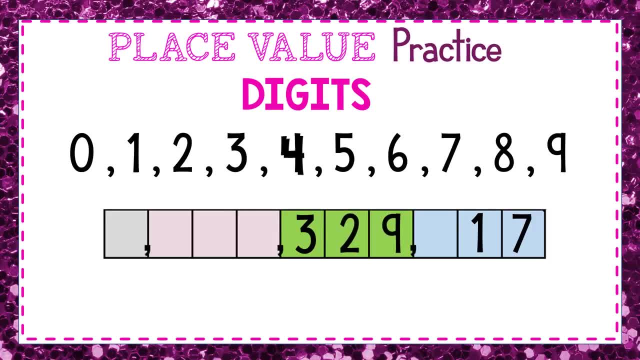 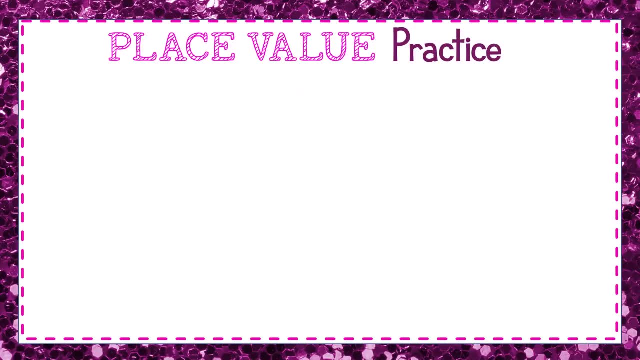 thousands place a nine in the thousands place, a four in the hundreds place, one in the tens place and a seven in the ones place, and these six digits make up this six digit number: three hundred twenty nine thousand four hundred seventeen. so now let's create a number being given these rules. let's create a: 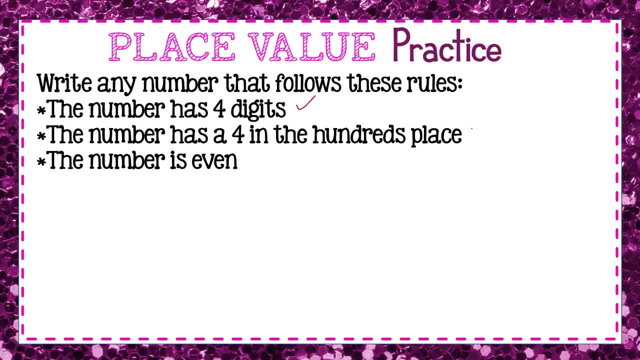 number that has four digits. the number has a four in the hundreds place and the number is even. so let's start with the four digits. my number that has four digits. I know I'm gonna need four spaces, so I'm going to start with that. you. I know that the number is going to have a four in the hundreds place, so my 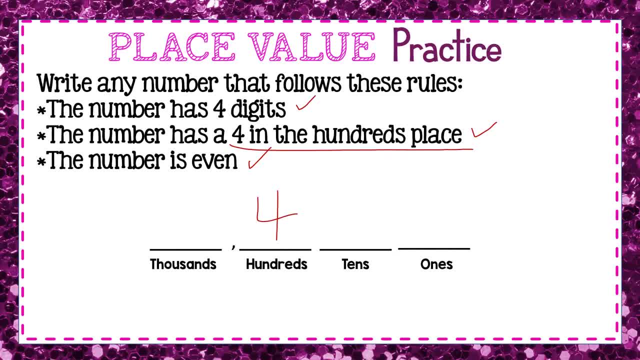 hundreds place is here and I'm going to place the digit four in that place, and this number is even. so, in order for a number to be even, I have to look at the ones place, and the ones place determines whether or not that number is even if 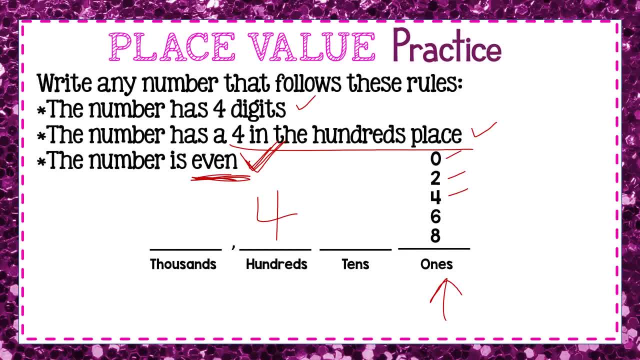 the ones place has a zero, two, four, six or eight in that place, then the number is even. so if I was going to write any number that follows these rules, as long as the hundreds place is a four and the ones place is an even number, I can put any digit I want to in the tens place in. 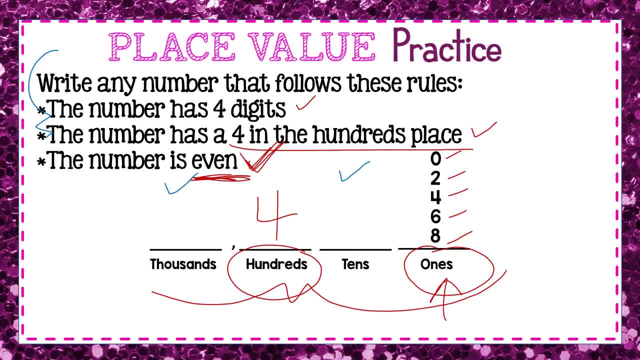 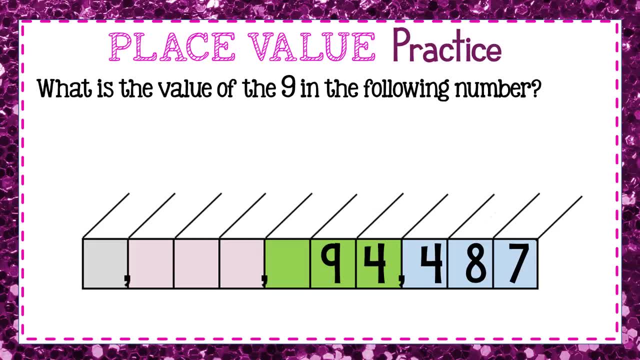 thousands place and it would still be answering this question correctly, because the number would follow the rules presented. so let's answer a question on a number. what is the value of the nine in the following number? ninety four thousand four hundred eighty seven. so, as you can see, the nine is here in this place. that is the. 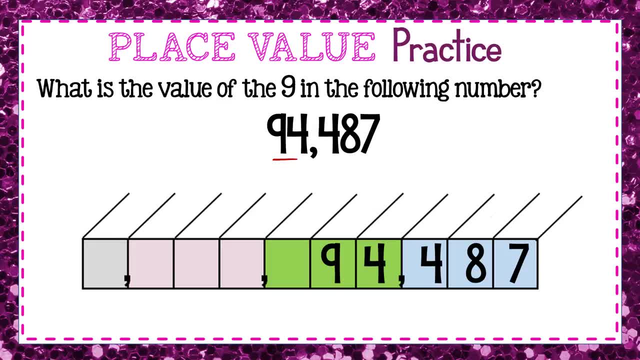 ten thousands place. and let's look at my place value chart. i see that that nine is worth ninety thousand because of the place that it's in. the four is worth four thousand. the four next to it is worth four hundred because it's in the hundreds place. the eight is worth eighty and the seven 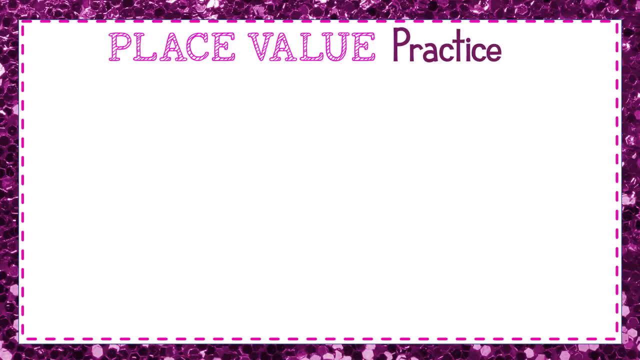 is worth seven ones. so there's two big things you have to do when working with large numbers and their place value. you have to be able to compare numbers and order numbers, you have to look at their value and decide which one's greater, less than or equal to, and you have to be able to. 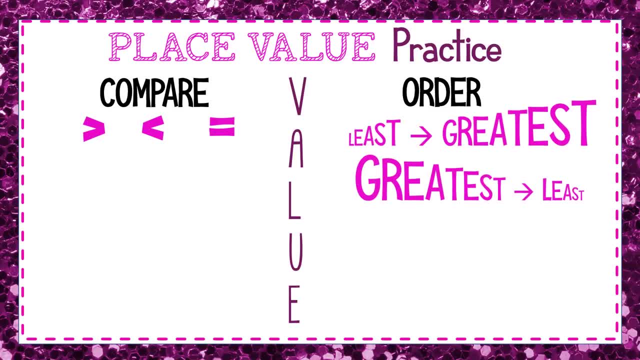 put numbers in order from, let's say, least to greatest or greatest to least. so let's practice comparing some numbers. here i have a comparison: 3206 is blank, then 3260.. so i tell my students to look at the first and the last numbers. and i'm going to look at the first and the last numbers. 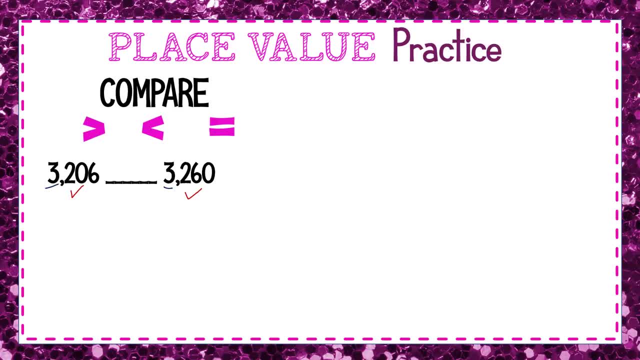 digit. three in the thousands place. three in the thousands place. does that tell me which number is greater, less than or equal to no, it doesn't. so i've got to go to the next place. i see i have a two in the hundreds place and a two in the hundreds place. that still does not tell me. 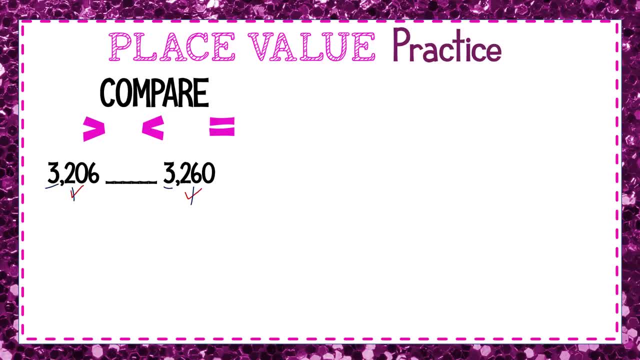 which number is greater or less than so. let's go to the next place: the tens place. zero in the tens place here, six in the tens place here. so six is greater than zero. therefore, 3206 is less than 3260.. so that's a true statement, a true comparison. 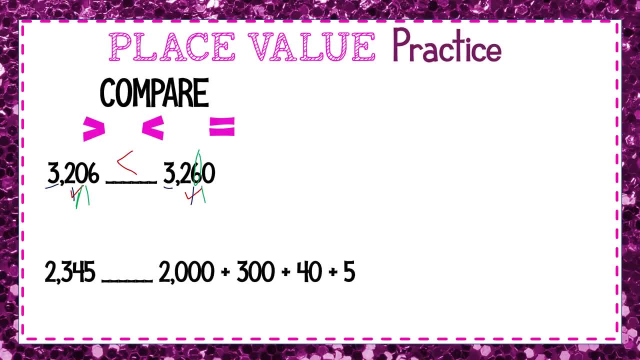 let's look at another comparison. so on this one you see that you have two thousand three hundred forty. five is blank, then two thousand plus three hundred plus forty plus five. so you can see that you've been given a number in expanded form and the number on the left is in standard form. so 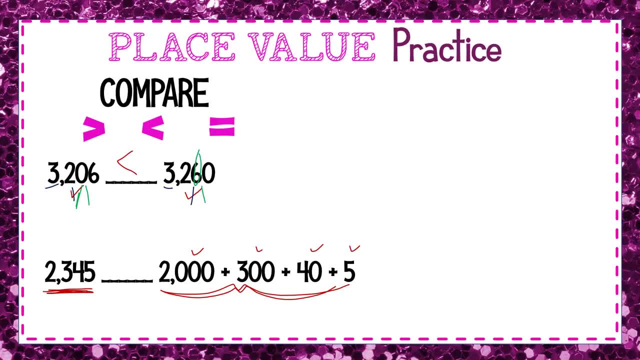 let's put this number in standard form. so i see that this number has four digits. i have a two in the thousands place, a three in the hundreds place, four in the tens place and five in the ones place. now these numbers are much more easily compared. 2345 is equal to 2345. these numbers were equal. so now let's talk about ordering numbers. 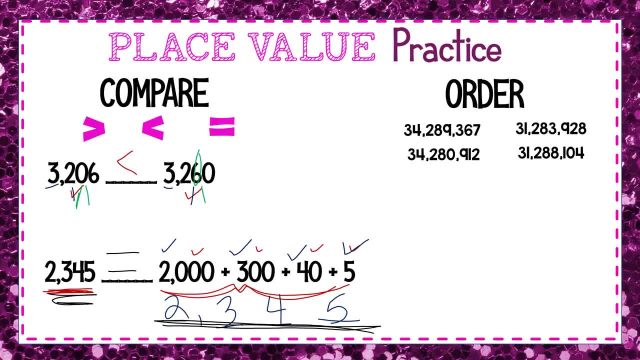 and here i have four large numbers that i'm going to order now. all of these numbers go up to the 10 millions place. these numbers are eight digit numbers, so let's do what i said before: let's look at the first digit to see which one is in order, and in this case, we're going to put these numbers in order. 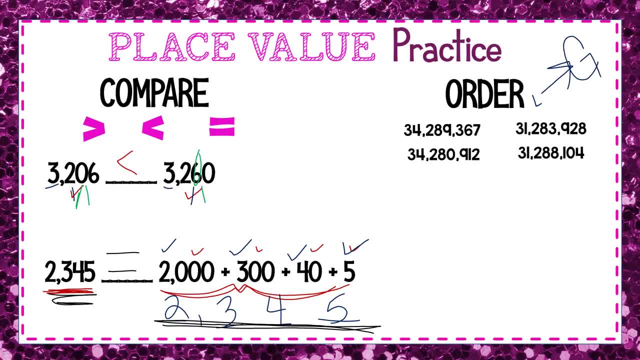 from least to greatest, and when i do this, i'm going to number them, with one being the number of least value and then four being the number with the greatest value. let's look at my first digit. i have a three in each of the ten millions places, so that doesn't. 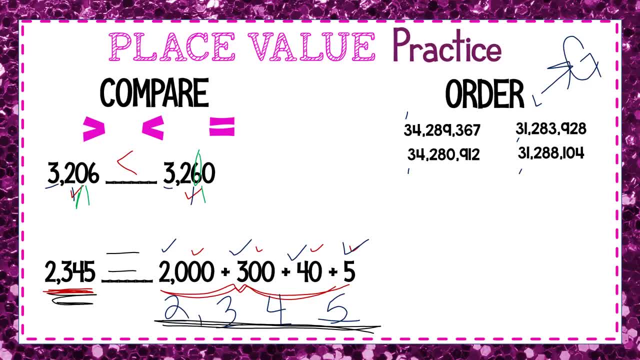 tell me anything of which one's greater or less. i see that i have a four in the millions place and i have a one in the millions place of these ones. so i know that these two are going to be my first two numbers. let's go to the next digit. so i see i have a two in the 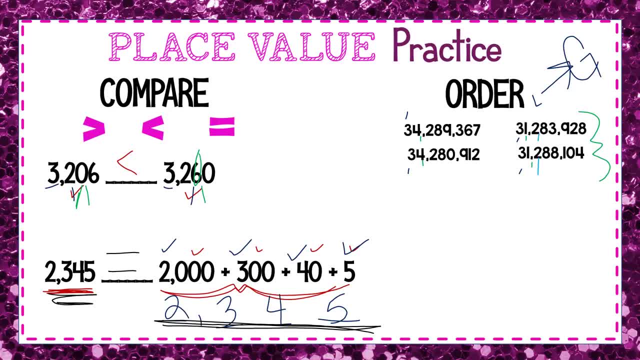 hundred thousands. two in the hundred thousands still doesn't tell me which one's greater or less. eight in the ten thousands still doesn't tell me what i need to know. three in the thousands. eight in the thousands. so this is my number of least value. i will put a one. 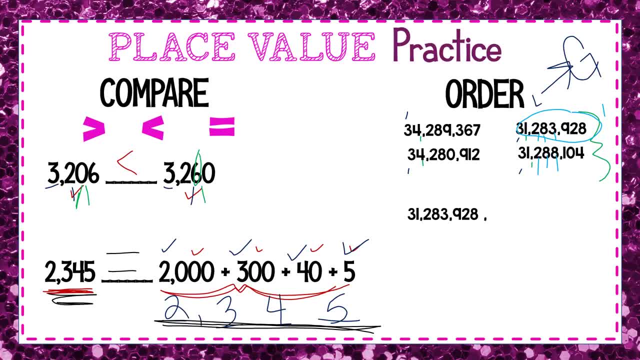 by that, that number is first in my list. 31 million 283 928 is my least valued number here, so i'm done with that one, and i already know which one's going to be next, because it's the one with a one in the millions place. so next is 31 million 288 104 and i'll put a two by that. so now i have these two.